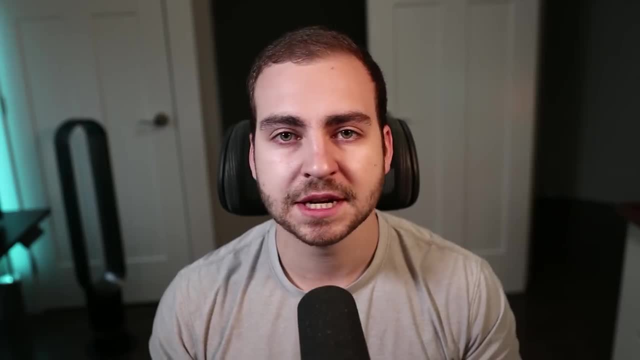 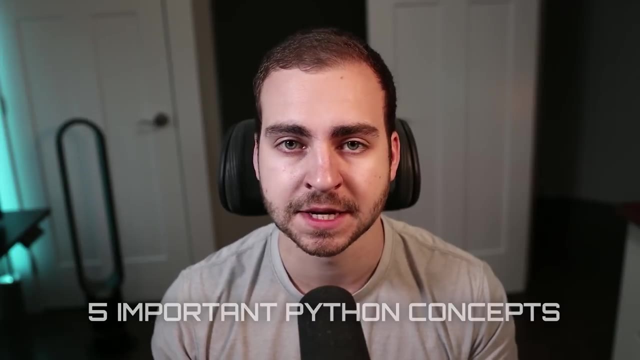 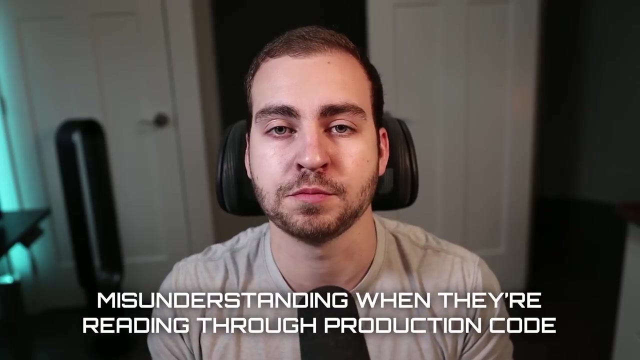 If you're interested in becoming a developer that writes any type of code in Python, then you need to understand these five very important Python concepts. These are what I see most beginner and intermediate Python programmers making a ton of mistakes with and misunderstanding when they're reading through production code. The goal of this video is to make 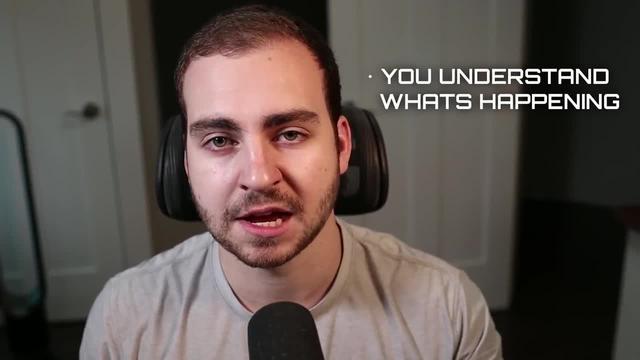 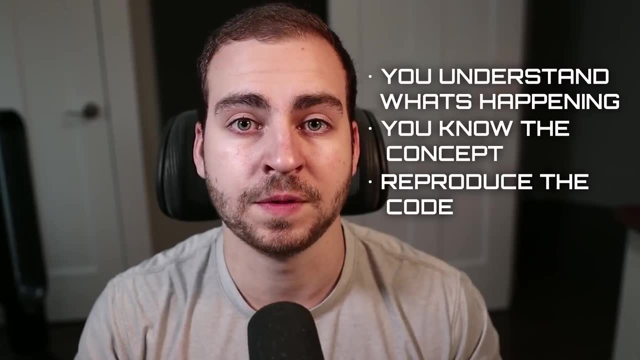 sure that when you're reading through production Python code, you understand what's happening, you know the concept and then you can reproduce that code and write your own pull requests and own features using Python code that other developers will understand and expect. So with 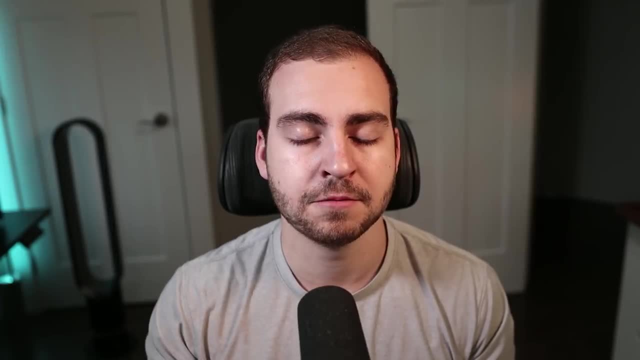 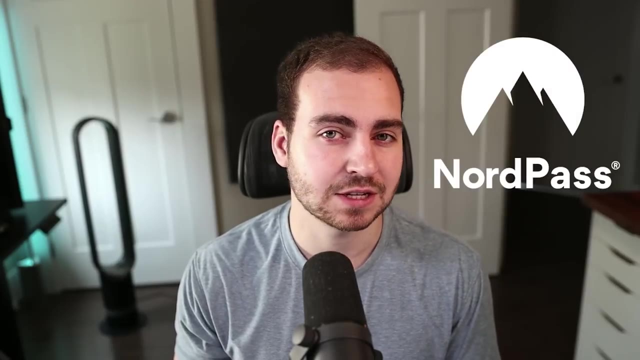 that said, let's get into the video. after I share with you the first very important concept you need to understand: which is the sponsor of this video: NordPass. NordPass is the ultimate password and credential management solution that I've actually been looking for for a long time Now. I don't 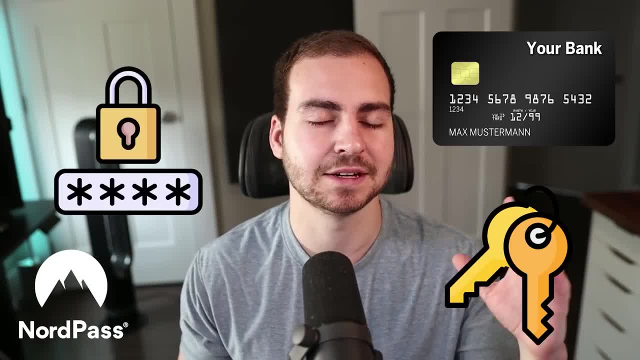 know about you guys, but I have a lot of passwords, credit cards, bank details, private keys, et cetera- And oftentimes I need to share these with my coworkers, making it a conversation. So I'm going to share a few of these with you guys. So let's get started. 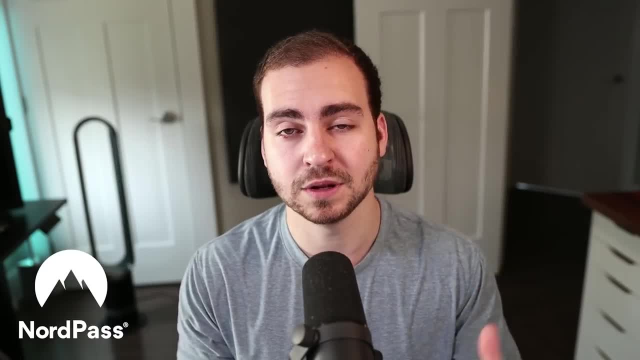 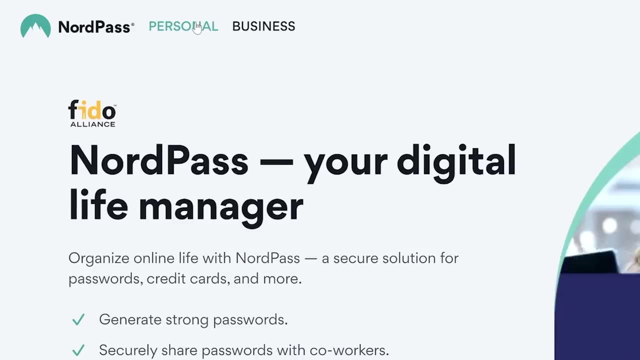 NordPass has a constant struggle to not only keep this data secure and safe, but to allow them to access it quickly without having to message me all the time. Now NordPass fixes this problem, because it allows me to store both my personal or my business data in a single secure location. 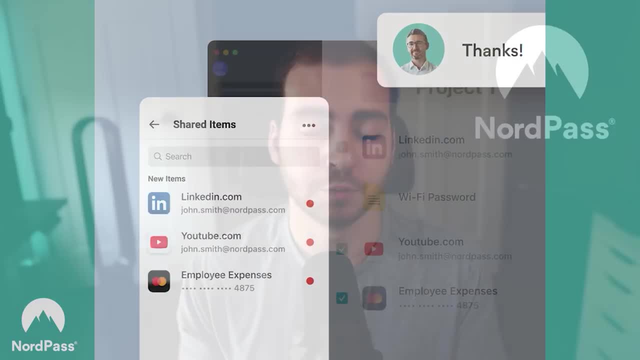 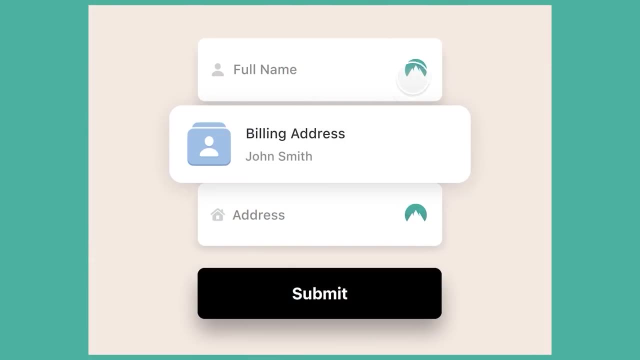 and then give different access to members of my team. Now, if you don't believe me, you can check it out from the link in the description and use the code tech with Tim, which means you'll no longer have to be sending messages or receiving messages. 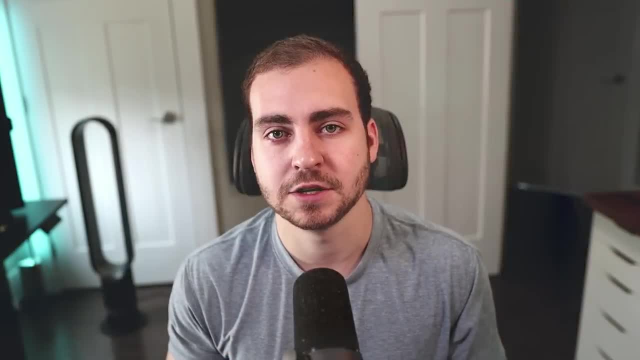 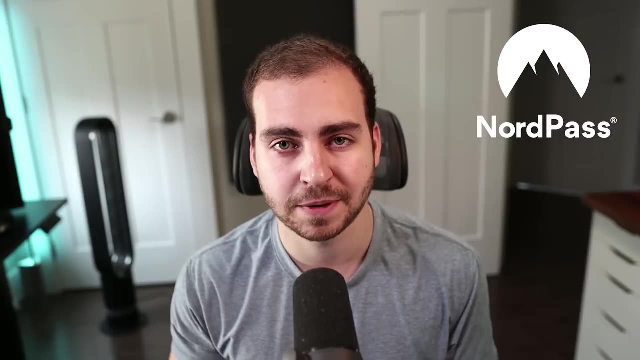 asking for passwords, Not to mention that NordPass has features like autofill, data, breach detection, an activity log, a password generator and much more. Check out NordPass from the link in the description and use the code tech with Tim for a three month free trial, So you can take. 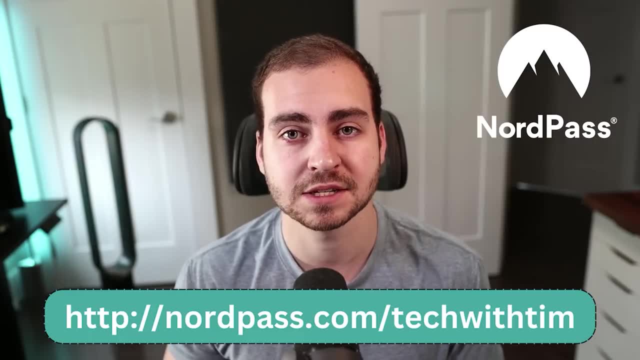 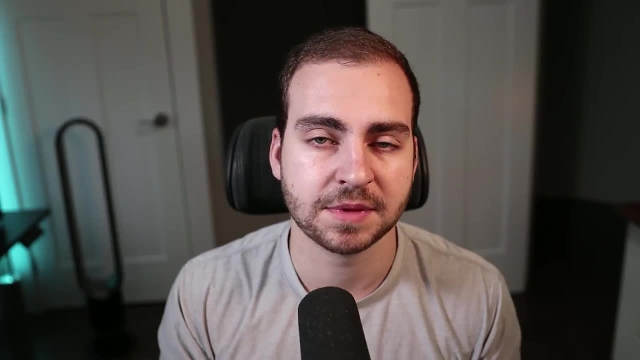 control over your data and your accounts. Thanks again to NordPass for sponsoring this video. So the first concept to go over here is mutable versus immutable types. Now this is the concept that most beginner and intermediate programmers make mistakes with. Don't worry if you already. 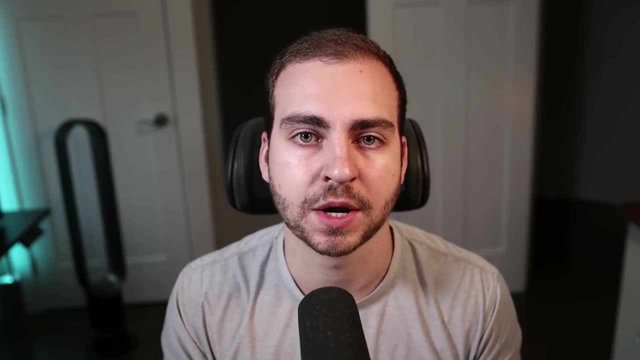 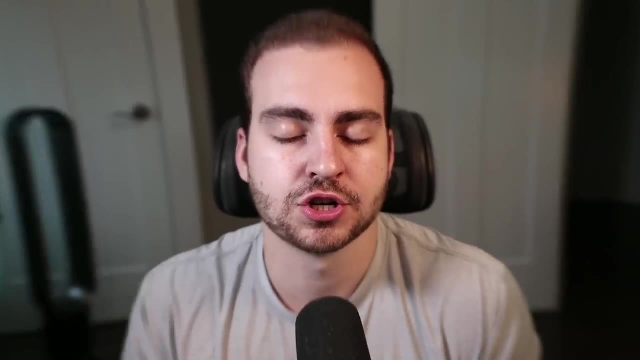 understand it. there's a lot more complicated concepts, So stick around for the rest of the video. Regardless, an immutable type is something that cannot change. A mutable type is something that can change. An example of these in Python is the following: So immutable types are going to be our. 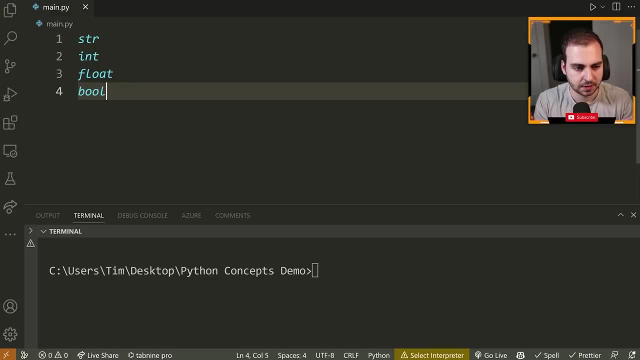 string, our int, our float, our Boolean, our bytes type and our tuple type. All of these are immutable meaning once you define this, you cannot change it. However, we have mutable types in Python, which are the list, the set and the dictionary And pretty much. 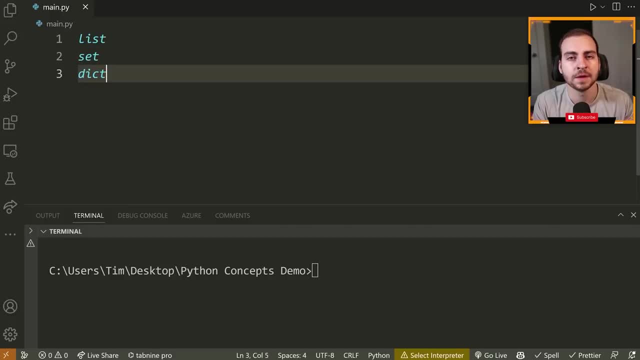 any other type used from some third-party library or module. these can change, which means once you define them, you can actually modify them. Let me give you a super quick example here of immutable versus mutable. Then we'll go into a more complex one using a function, which is where I see most. 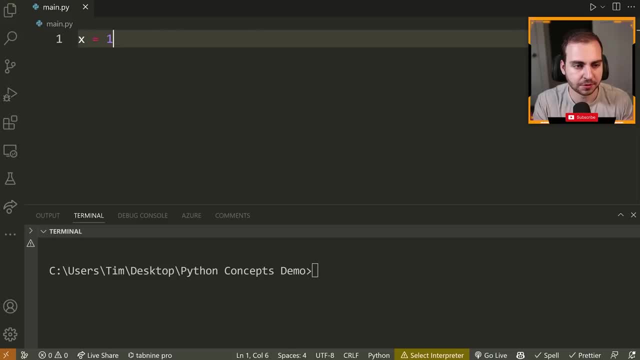 beginners make a mistake. Okay, So let's say we have some number like X equals one and we say Y is equal to X And in fact let's change this to a tuple which, remember, is immutable, meaning we cannot change it. Actually, to quickly show this to you, 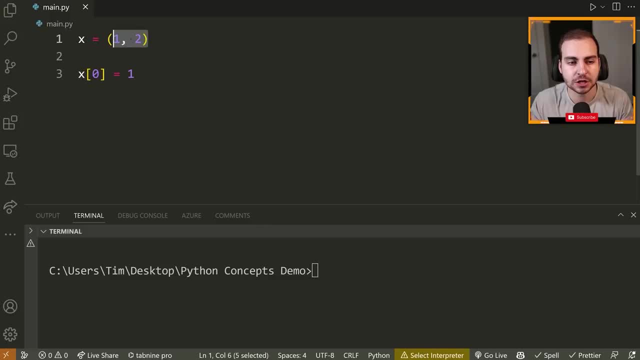 try to do something like X- zero is equal to one, where we're trying to change this tuple without reassigning something to this variable. So if I go here and run my code, notice I get an error and it says the tuple object does not support item assignment. Now the reason it doesn't support: 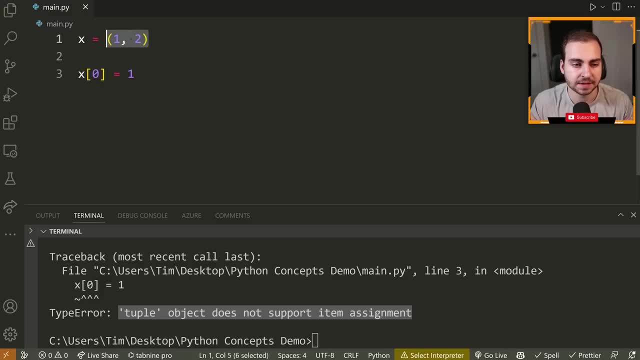 that is because this is immutable. That means that once I define this tuple, I cannot change it. Now, if we go here and do something like Y equals X and let's come and say X is equal to one, two, three, I just want to show you if I 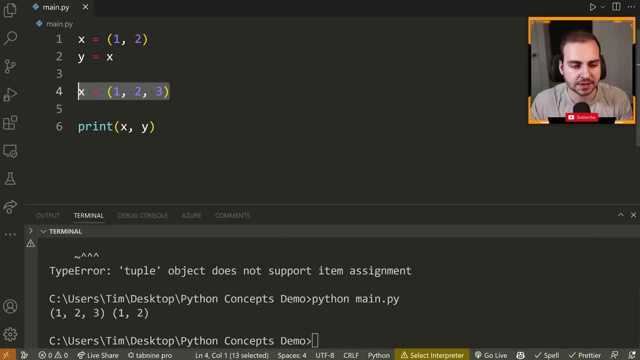 out both X and Y here, that my change to X here after assigning X to Y did not affect Y. The reason for that is whenever you're using immutable types, when you do an assignment to another variable, So I do something like Y equals X, it makes a copy, So an actual, real copy of this immutable object. 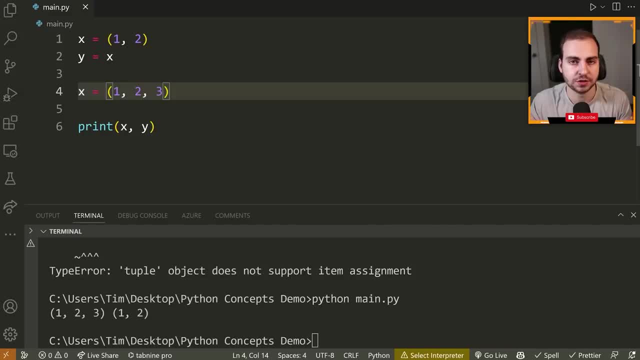 meaning that if I now go something like X is equal to one, two, three, that's not going to affect Y, because I'm not modifying what Y is storing. I'm just reassigning a new value to X. I know that seems trivial, but the reason I'm illustrating this to you is because this works. 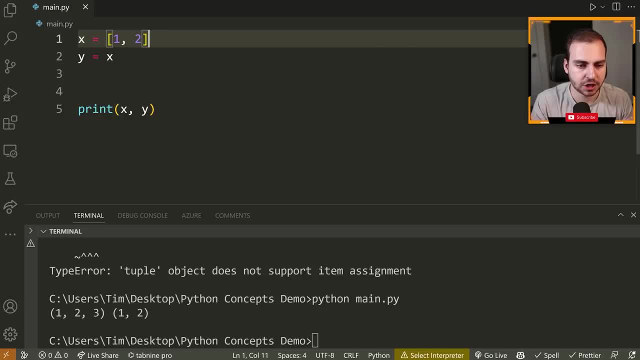 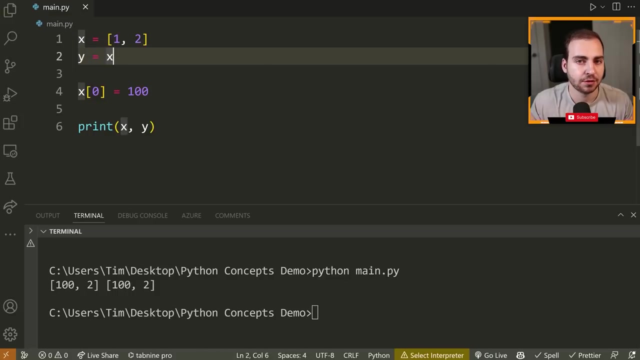 differently when we change this to a list. So if I change this to a list now and then I come and do something like X, zero is equal to 100, you might think that Y is not going to change, But when I run this, you see that both X and Y have the same value. Now, the reason for that is when you're 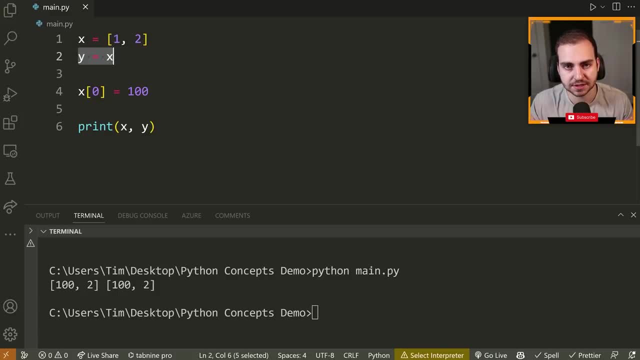 using mutable types and you do something like Y equals X here, So you're signing a variable to another variable And this variable is storing a mutable type. What happens is you actually store a reference or an alias to this same object, meaning that if I make a change to the object, like I'm doing right here, it changes. 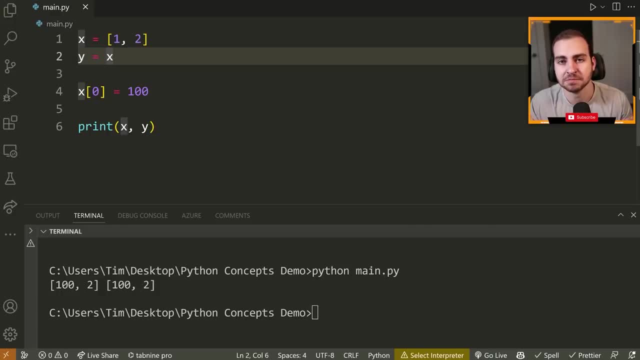 for both of these variables because they're actually storing the same object. In fact they're storing a reference to the same object. So, again, if you change the underlying object, then it changes for both X and Y. That's the difference between immutable and mutable types. 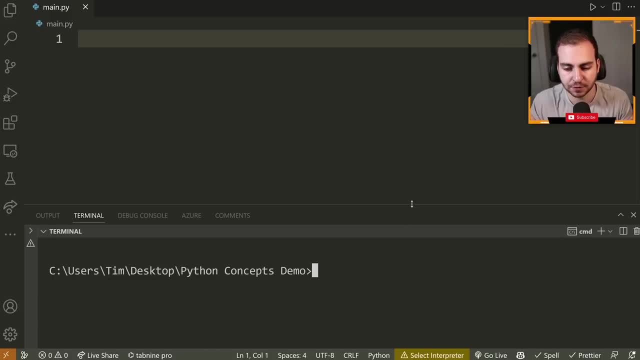 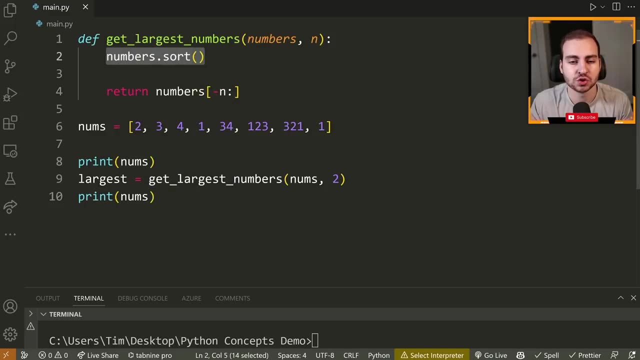 Now let me just paste in a quick example here that will illustrate this even a little bit further. You can see in this example we have a function that returns the largest numbers. It returns the end largest numbers. Actually, what it does is it sorts the list of numbers that it accepts. So what I've done down. 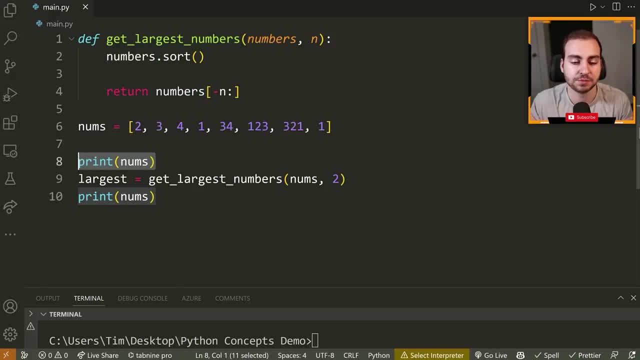 here is: I've created a list of numbers. I printed out what the value of the list was before I called the function And then I printed out what the value was afterwards. Now take a guess, if you want, at what you think the output's going to be. but I'll go ahead and run the code And you can. 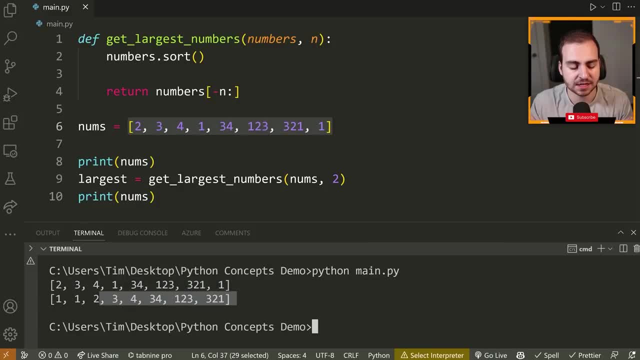 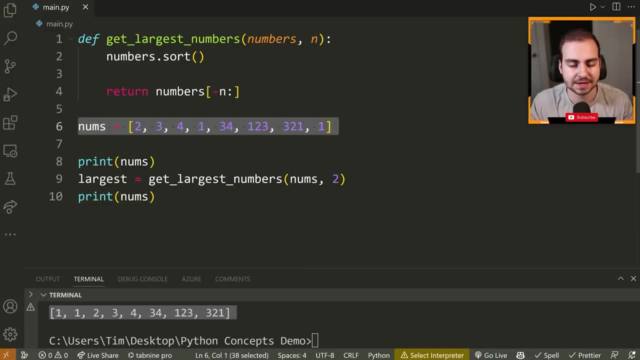 see here that we actually get the list before that's unsorted And then the list becomes sorted afterwards. Now the reason this occurs is because what happens is we're going to have a function that when we call this function, we pass this nums list as the parameter numbers. Now, since we're 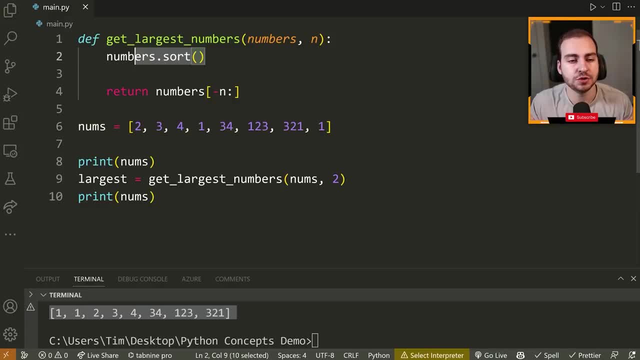 passing a mutable object. a list is mutable. When we do a numbers dot sort, what this does is actually sort the list in place. Now numbers here is going to be storing a reference to this same list. So when I sort the numbers parameter here, since I had passed in my numbers array, it ends. 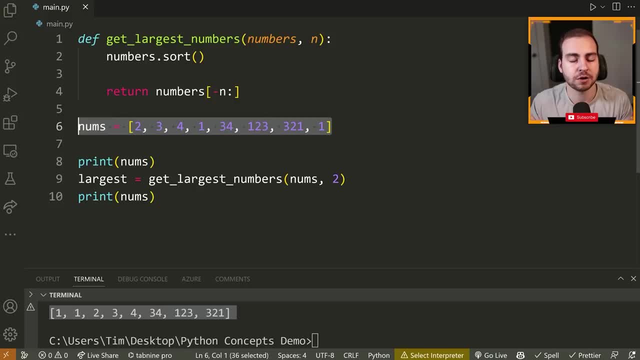 up sorting that numbers array That's down here Seems a little bit strange, but the reason this is going to happen is because we're using a mutable object. So the point here is that you need to understand when you're using mutable versus immutable objects, because you can have functions. 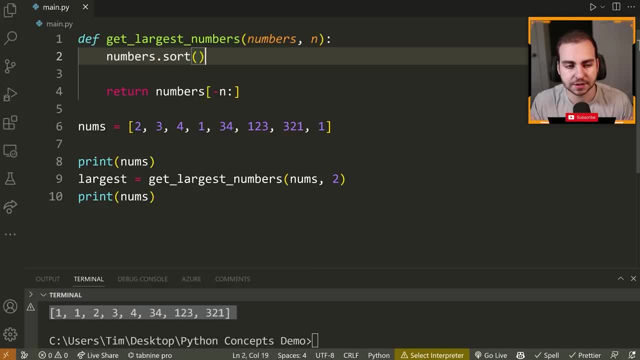 like this that can perform side effects on your mutable objects. This is referred to as a side effect because what happens is one of the parameters is being mutated or modified inside of the function. Sometimes you want that to be the case, Sometimes you don't want that to be the 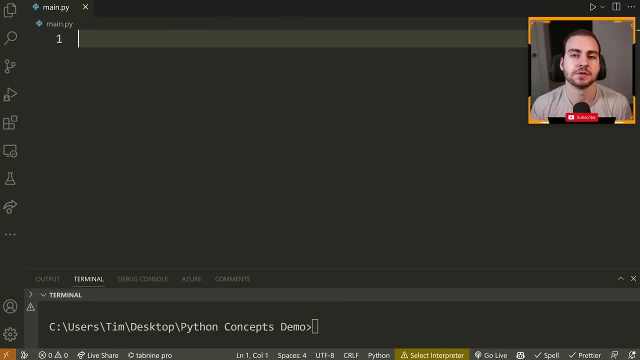 case, You need to be intentional when you're writing your code. So the next concept to understand here is list comprehensions. Now, the reason you need to understand this is because it's used Quite a bit in Python And oftentimes you'll see people writing fairly complicated comprehensions. 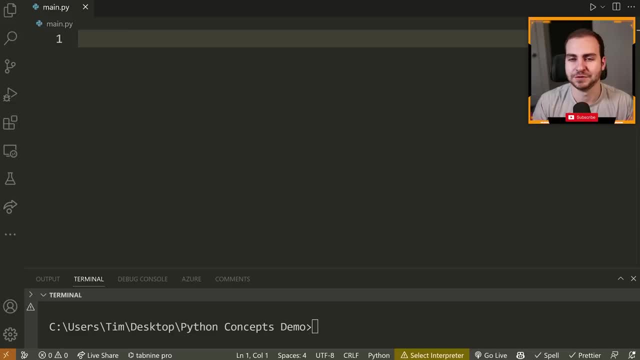 to simplify a line of code. Now this can kind of do the reverse. Sometimes it can actually make it more complicated. Regardless, you need to understand what they are so that you can actually understand them if you see them in some production code. So let's have a look at a list. 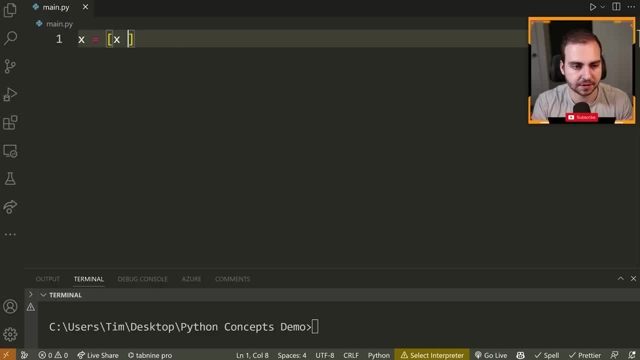 comprehension. So the most basic comprehension you can do here is something like X, or we'll go with I for I in range, and then maybe something like 10.. And in case you had to guess it here, what this is going to do is give me an array that contains the numbers. 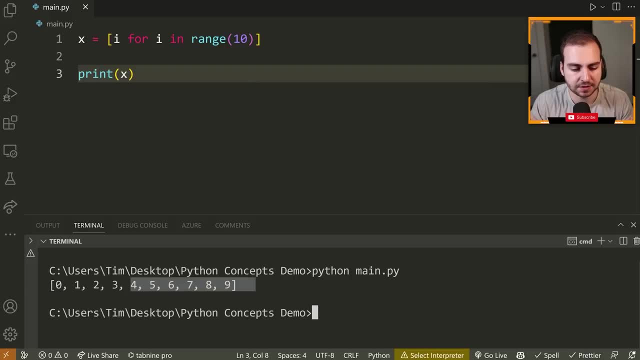 zero through nine. So let me open up my terminal and run this and there you go: We get zero through nine. So this is a list comprehension where essentially you write a for loop inside of a list. What you do on the left-hand side is you put the value that you want to populate the list. 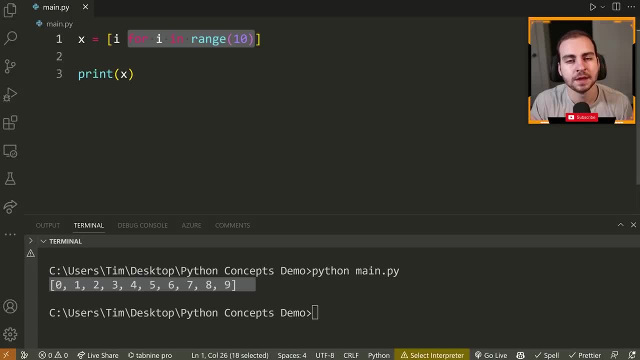 with, and then you have some kind of iterator. In this case we have a for loop that's going to loop through and generate these different values. Now, this is a very simple list comprehension. You can make much more complicated ones. For example, we can have a: 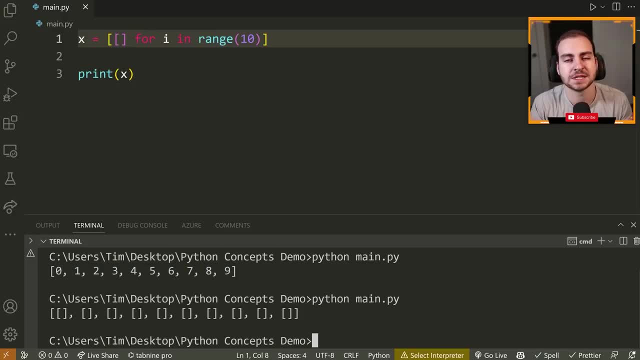 list here instead. So now if I do a list, we have a bunch of empty lists inside of this list. But just like we have a list comprehension here, we can have one inside of this list. So I can do something like for: so actually, let's go with J for J in range five like that, And now we have. 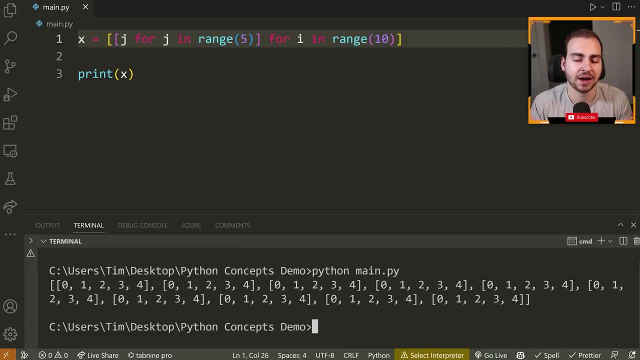 a nested list comprehension. And if I run this code, you can see that now we get a bunch of lists that contain five different values, inside of them 10 times Okay. So that's one thing you can do. Another thing that we can do here: 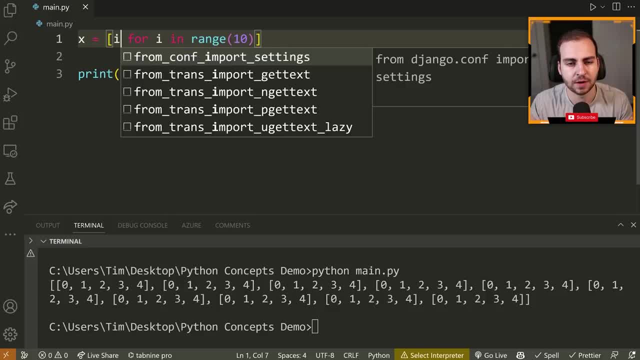 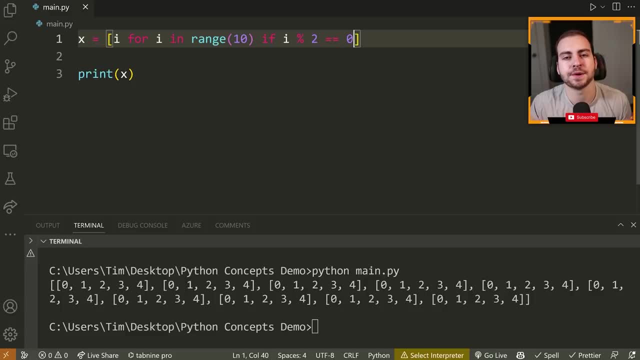 is the following: So let's go here and say I for I in range 10, and then we can put in if statement and we can say: if I mod two is equal to zero, Now this means we're going to only put. 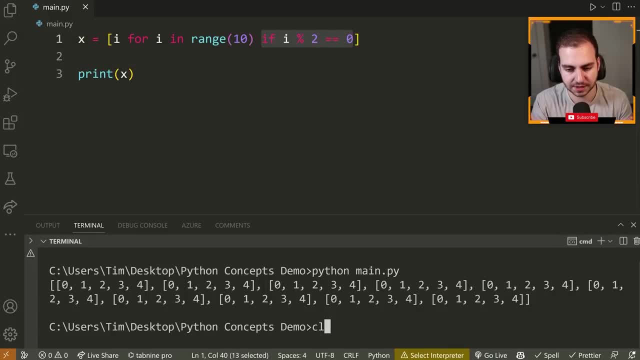 this value here If this condition evaluates to true. So in this case we're only going to put even values or zero inside of this list. So when I run this, you see that we get all of the even values up to, but not including 10.. All right, So the next concept here is the different Python. 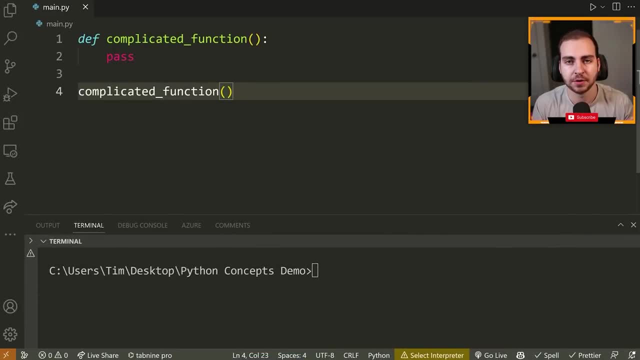 argument and parameter types. So there's quite a few. That's why I'm going through this concept And a lot of times people have no idea what they are beyond the basic ones. So if we define a function here like complicated function, we can have what's known as our necessary parameters or our positional 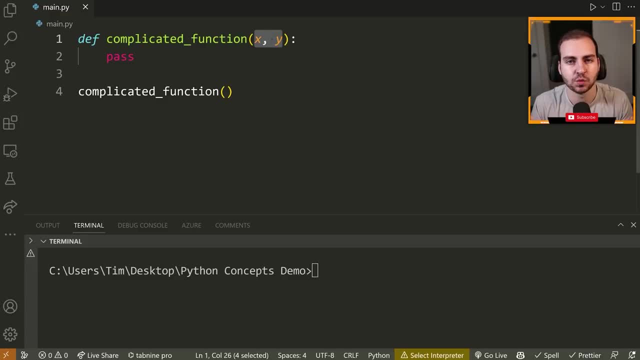 parameters that are defined in order, So I can have something like X, Y. Now, these are required and they are positional, meaning that if I want to pass values here I have to do something like one, two, right, I pass them in the order in which I want them to be kind of assigned. So X is one. 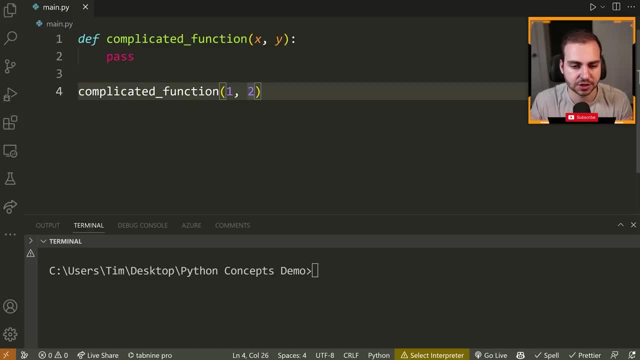 and Y. However, I can actually switch things up a little bit here, And as I pass these arguments, I can do something like: Y is equal to two and X is equal to one, And now, if I go here and print this, so X and 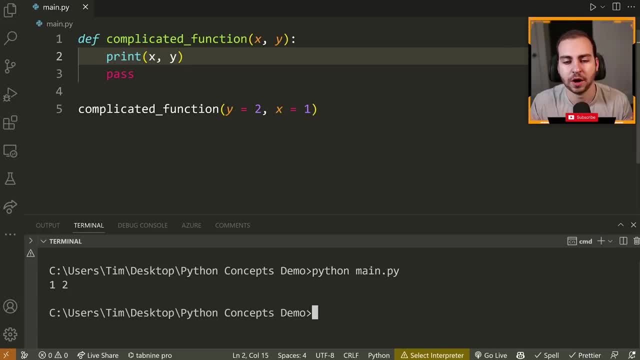 Y, you see that we get one and two. So this is valid. when you are calling a function, you can actually write out the name of the parameter, whether or not it's positional, optional, et cetera, And then you can just assign it directly inside of here. This allows you to no longer. 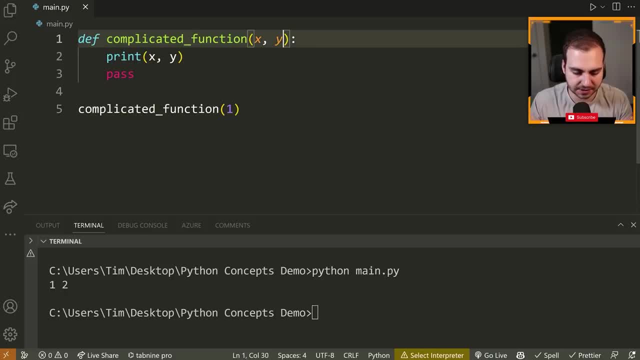 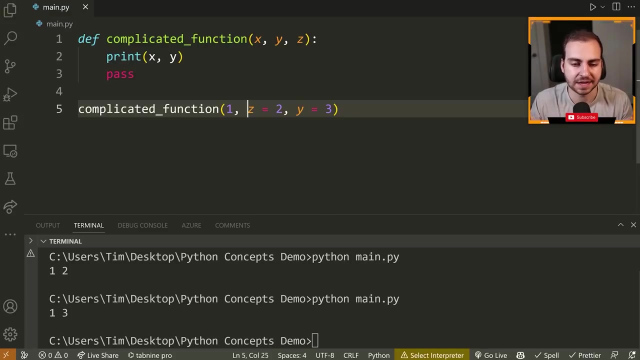 pass this positionally. However, if I pass some positional arguments- so let's say I do something like one Now- I can do something like: Zed two, Y is equal to three. So I can pass some of the arguments positionally and then some of them I can pass, uh, using the kind of keyword argument. 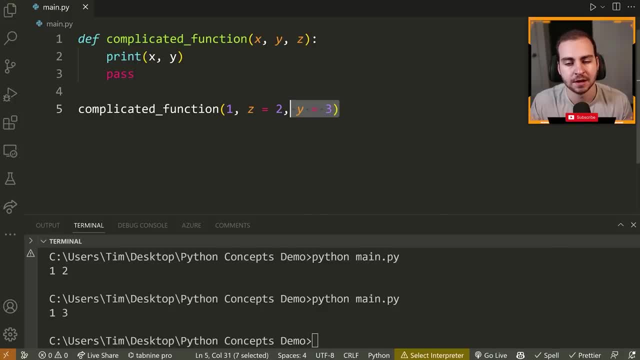 here, or you know, the named argument, whatever you want to refer to it as. by the way, inside of your function call, you refer to these as arguments and up here in your function you refer to these as parameters. So I just wanted to show you that I can pass some of these arguments, So I can pass. 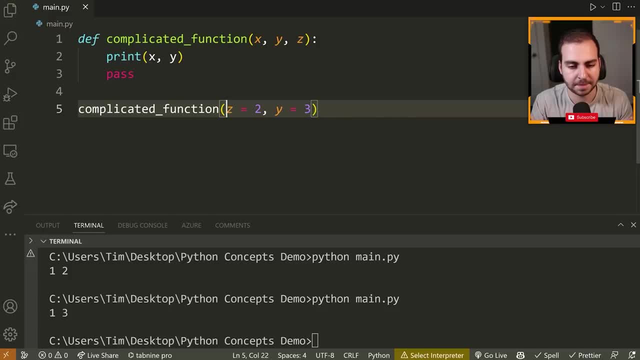 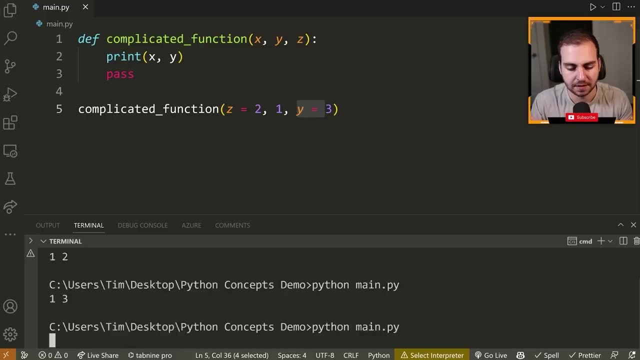 these positionally. However, things get a little bit weird If I try to pass some positionally and some using the keyword. So in this case I have like Z equals two, one and then Y equals three. If I try to run this notice, I get an error and it says a positional argument follows a keyword. 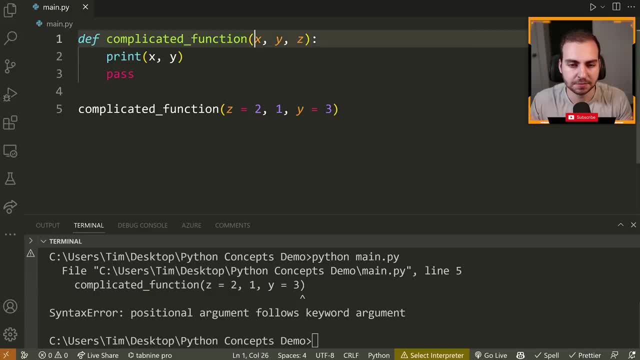 argument, which you're not allowed to do. So if I want to use some positional arguments and the rest keyword arguments, that means that I need to start by defining my positional arguments. Then I can do the keyword arguments after. hopefully that's clear. Uh, but that was the first thing to 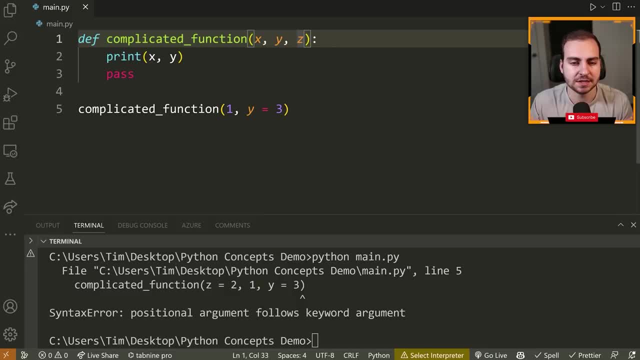 go over, Okay, Okay. Next thing is optional parameters. So inside of your function you can mark one of your parameters as optional by putting an equal sign. So if I do, Z equals two, in this case none. Now, this is optional, meaning I'm not required to pass it when I call this function. So if I call with one and 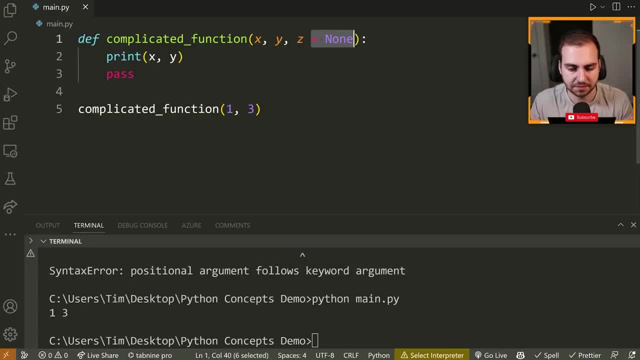 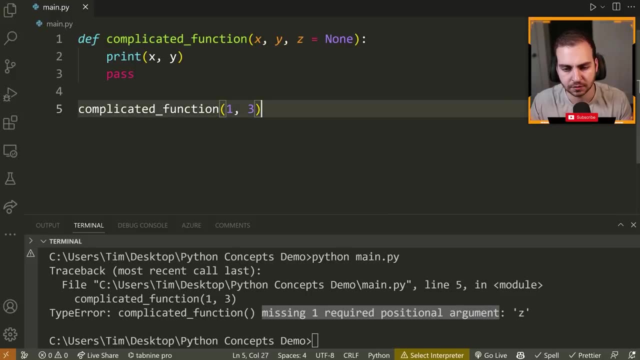 three here you can see this is perfectly fine. However, if I got rid of the equal sign here, so I made this no longer optional, then I get an error and it says it's missing one required positional argument. Okay, That's worth noting. Now, if I try to access Zed here, 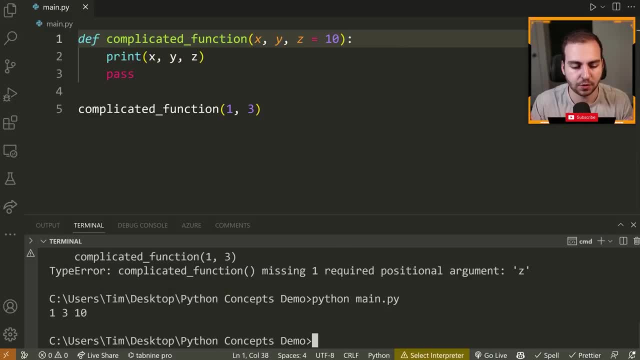 you'll see that actually, let's make an Eagle with something like 10.. If I run this, it actually gets its default value. So when you make something optional, really what you're doing is providing a default value for it. which means, if you don't pass that value, when you call the function by, 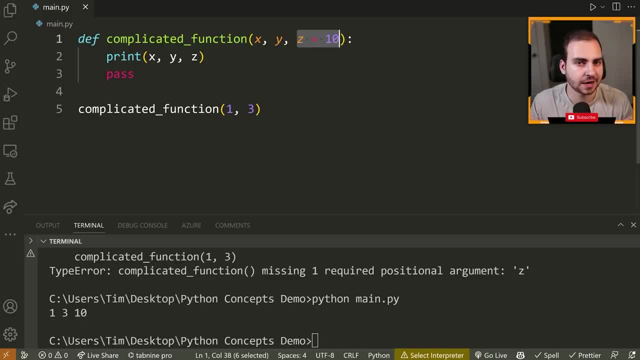 default, it will be equal to that value. Okay, So that was actually the easy stuff. Now we move on to the more complicated ones. Now we have something referred to as Asterix arcs. Now what this allows us to do is actually accept any number of positional arguments. So I 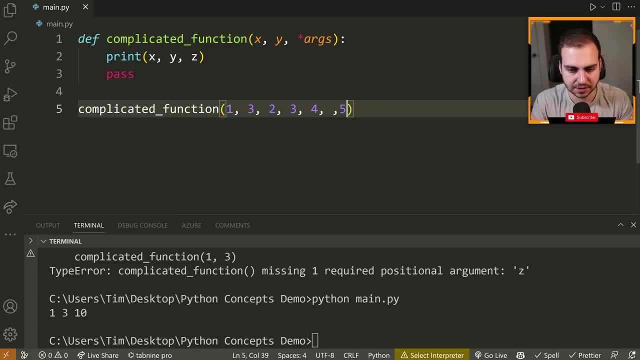 I can pass a bunch of arguments like this. Okay, I can pass no additional arguments. I can pass one to whatever it's any number after my positional arguments. So if I print out X, Y, Z and then args here and I run the code, you 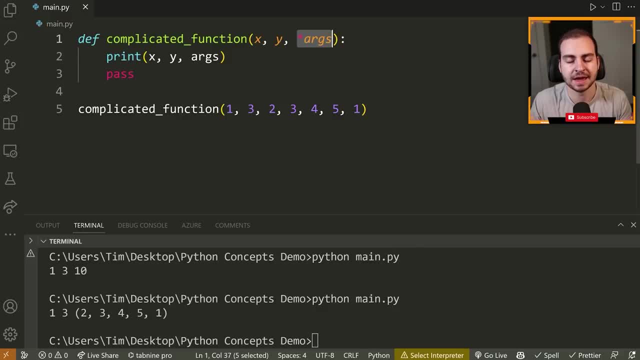 see that this is perfectly valid. So when I do this, asterisk args again. this means okay, I'm going to accept any number of positional arguments at this point. So after my two positional arguments that I have here, and then it's. 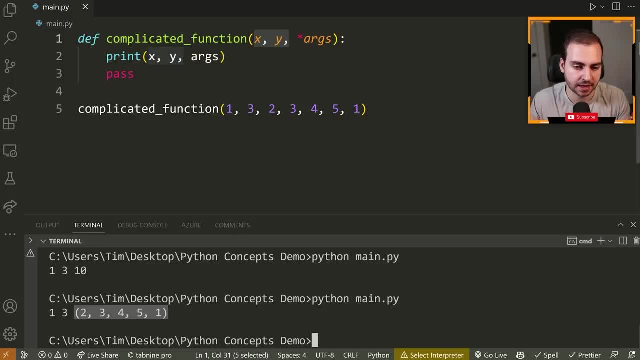 going to store all of them in a tuple which is an E mutable type. Okay, If we just have star args here, then you see it works the exact same way. We accept any number of positional arguments, even zero right. So 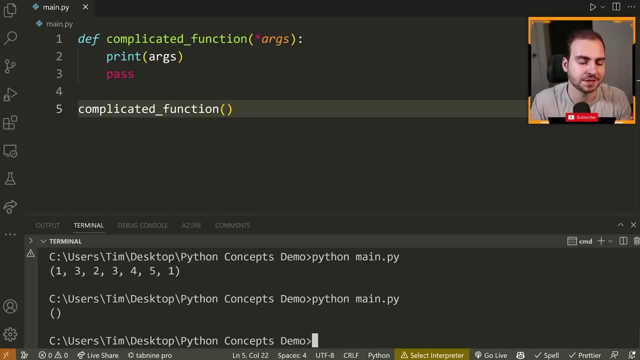 if I have none here, this works perfectly fine. Okay, That is star args. Now we also have star star quarks. So when you have star star quarks, this means we're going to accept any number of keyword arguments. So let me 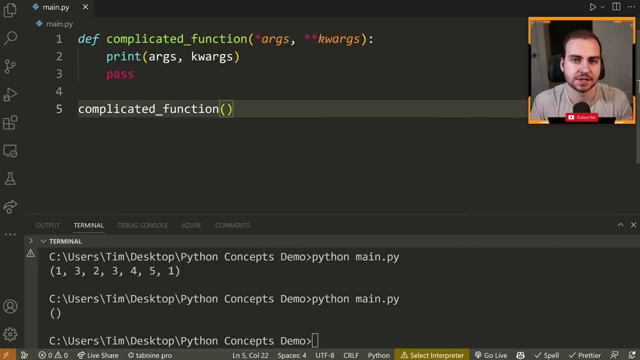 just print out quarks here and go and pass some keyword arguments. So the keyword arguments are like this. Some of them are like: X equals one, S is equal to I don't know, Hello. B is equal to true. whatever Let's do, 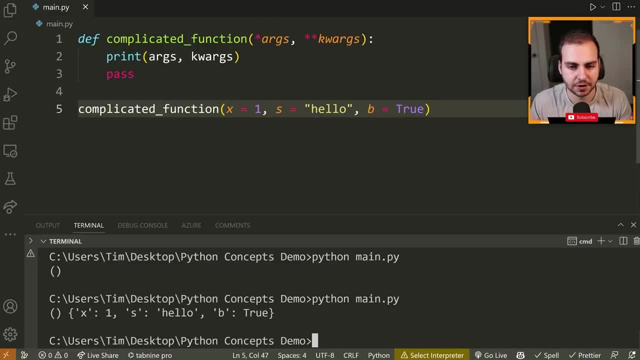 a capital, true here. So now, if I run this, you see that we have no positional arguments, but we have these three keyword arguments and they are stored inside of a dictionary. So if I want to access any of these individual keyword arguments, I go quarks. 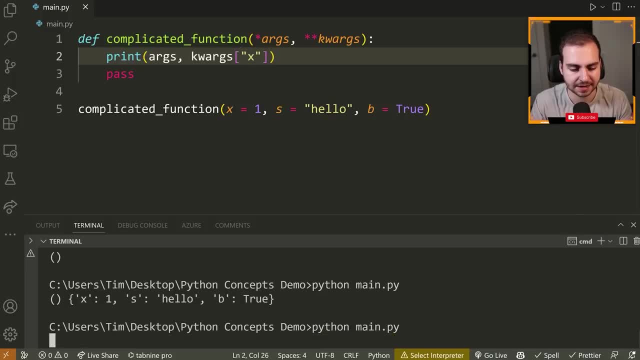 and then I reference whatever the key is. So I want to reference X here and notice I get one. Okay, This is useful when you want to make your functions dynamic. So I'm going to run this and say, okay, I'm going to make this. 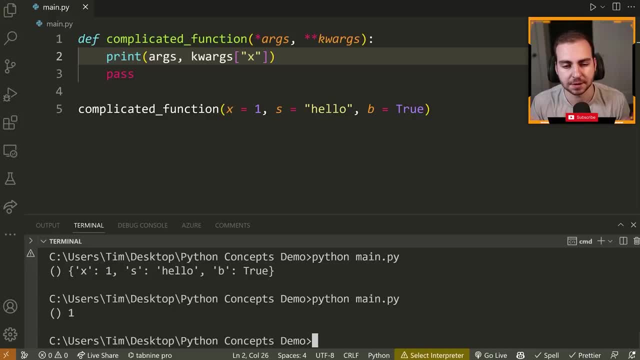 dynamic and you don't know how many regular arguments or keyword arguments you're going to be accepting. Now you can obviously pass both. So if I do something like one, two, three and then some keyword arguments here, you'll now see that we'll get. 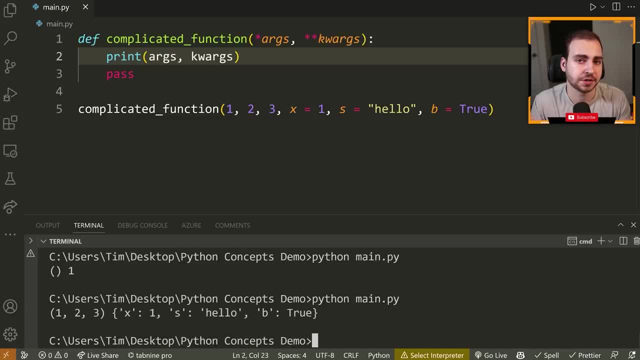 both args and quarks having some values, And then we can process those values However we see fit. Okay, Great. Last thing to show you is how to use these uh with inside of your function. So let's swap this round. 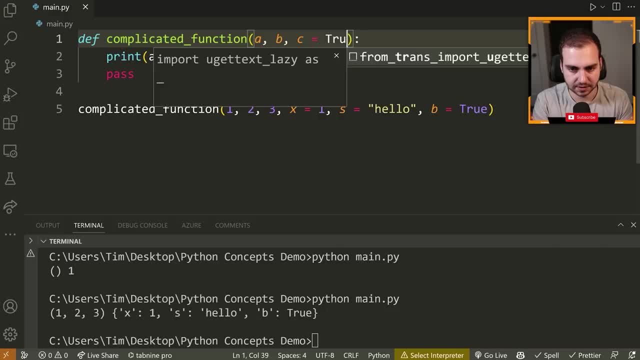 out and let's say we have like a, B, and then C is equal to true, D is equal to false. Okay, Now if we go here, we can actually use the asterisks to kind of break apart a list and pass different positional arguments. So 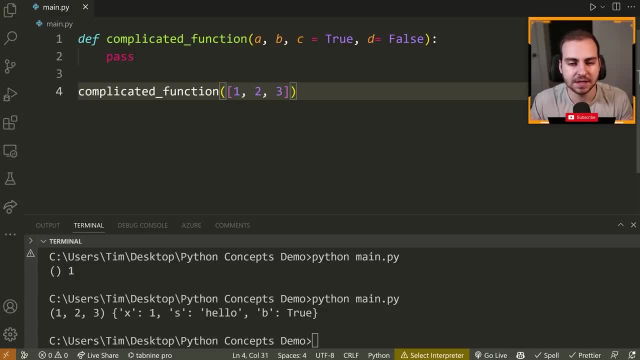 let's say, I have a list here and I have one, two, three inside of it, And these are actually the corresponding values for both a, B and not C, just a and B. If that's the case, I can't just pass this list, because if I do, 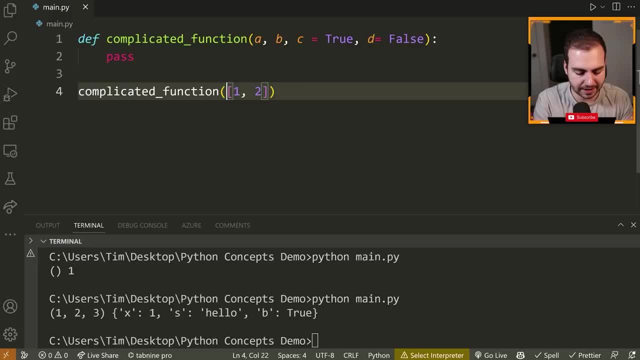 that it's going to be the positional argument for a. so what I can do is put an asterisk before it, And this is actually going to kind of decompose or break this apart into two individual points: Positional arguments. So if I go here and I print: 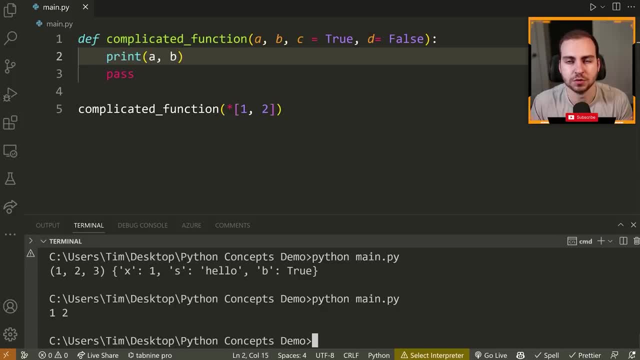 my a and my B and I run this notice- I get one. two works perfectly fine. Okay, Now we have the same thing we can do with our keyword arguments. So let's say I have a dictionary that contains my keyword arguments. Something like C is I. 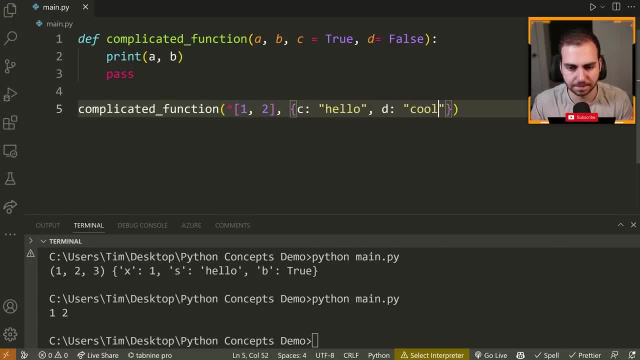 don't know. hello And D is cool. I can actually place a dictionary here and then put two asterisks before it, And what this will do is break this dictionary into its keyword arguments and pass it. Pass that to the function. So now I can. 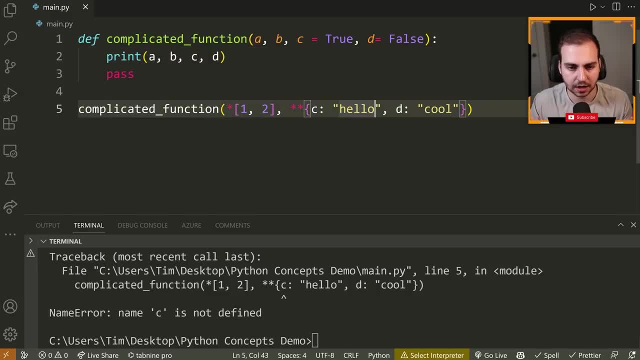 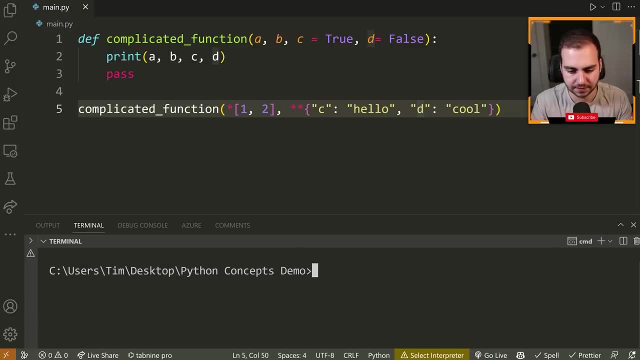 print C and D. And when I have a look, uh, what does it say here? C is not defined. Sorry, We need to just add a string here. Always forget that you need to do that in Python. Let's clear and 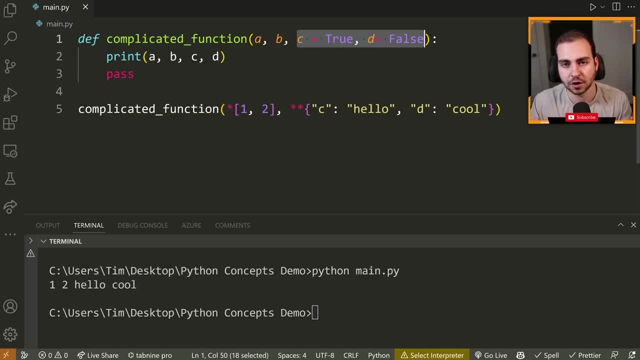 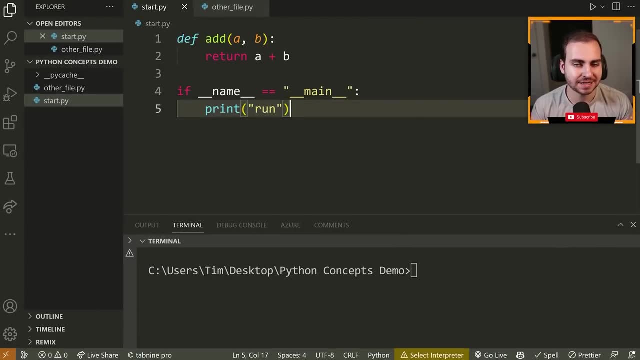 rerun and notice now that we get the values for our keyword arguments. So the next concept here is: if underscore underscore name equals underscore underscore main, Now this is simply telling you, if you ran the current Python file, the reason why it's important to 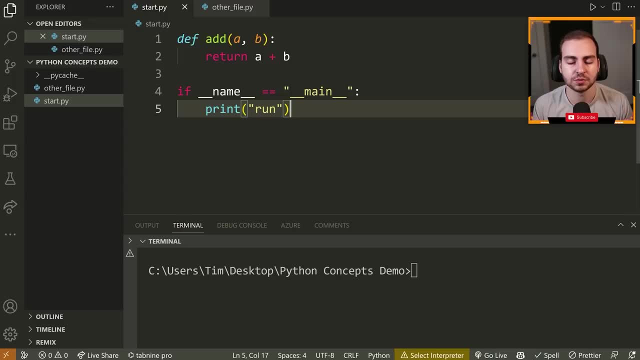 understand. that is because a lot of times you can have a bunch of different Python modules and sometimes you run the module directly. Other times it might be imported by a different module. So let's have a look at this example. In this case we 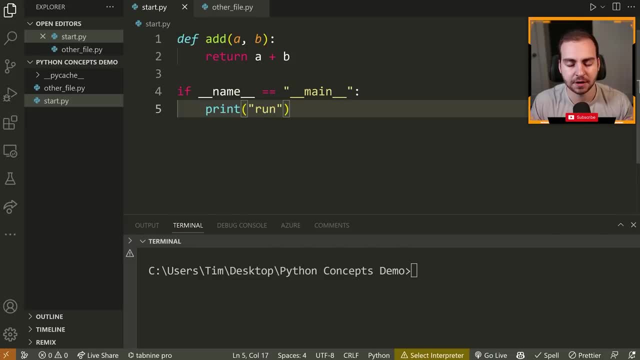 have startpy, We have some function, and then we have this: if underscore- underscore name equals equals underscore, underscore main, we're printing run, Then we have another file here. inside of this file We import the add function from this start module. Now, if I didn't have this, 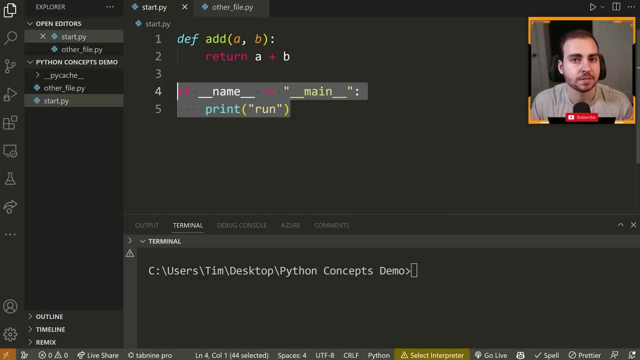 line here. what would happen is, when I import this module by default, Python would read the entire kind of block of code here, the entire file, And if I didn't have something inside of the if statement, so I just had say print run here, then 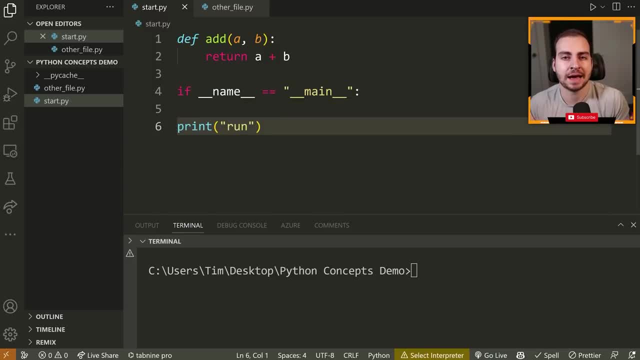 it would actually execute that line of code, which I might not want to happen, unless I'm actually inside of that module, or sorry, none side of that module. But if I ran that module, it's better if I just show it to you. So if I 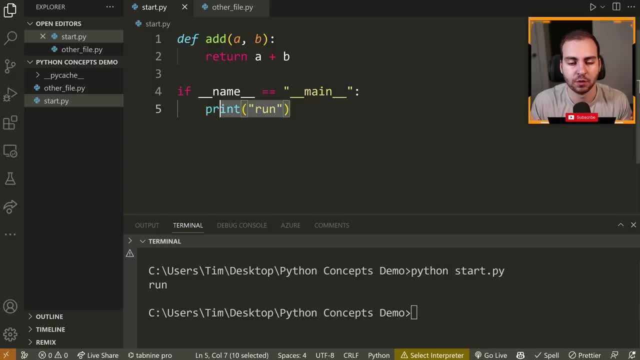 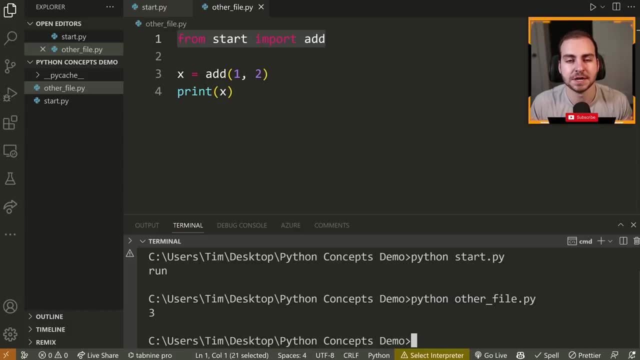 go here and I run Python startpy. you see that we get run printing out to the screen. However, if I run my other file, so Python other filepy, notice it doesn't print out run. However, if I remove this line here and 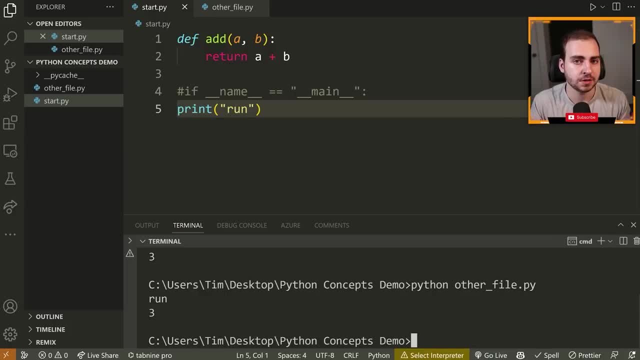 we remove the indentation now it will print run. So the purpose again of having this line is to determine if you ran this file directly. A lot of times you have a file where it has a ton of utility functions that are going to be imported. 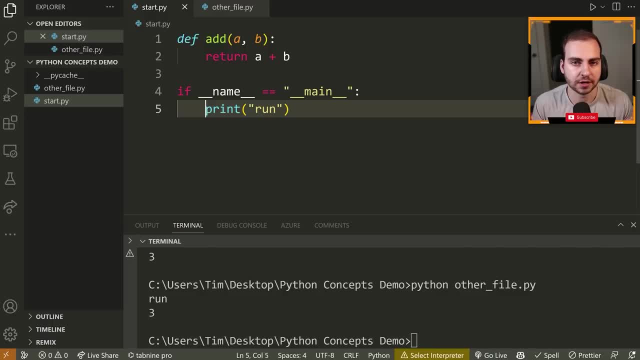 by other files, And then you have something you might want to do when you're running it directly, like maybe initializing a game or starting some program or sending an API request, whatever it may be, but you don't want this event to occur. You don't want. 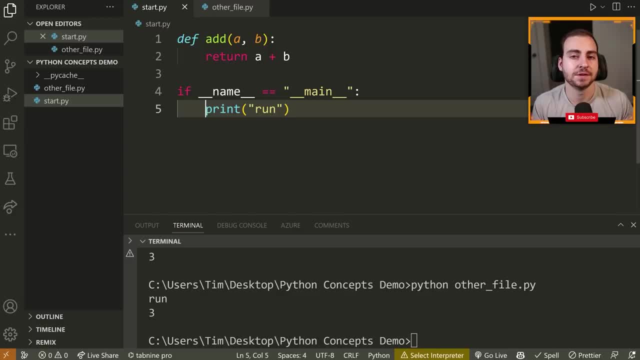 this code to run. So you run if it's being imported, uh, only if it's being ran directly. So that's how you use this. It's pretty much all you need to know. hopefully now you know. so the next. 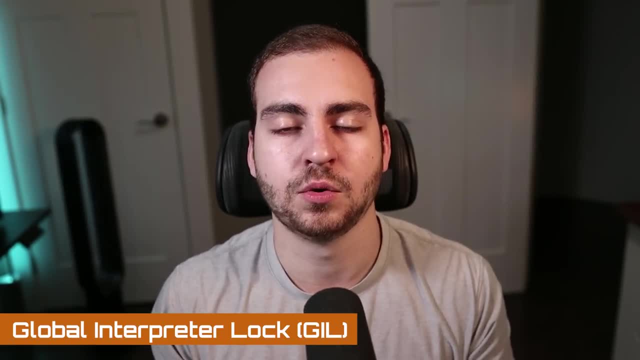 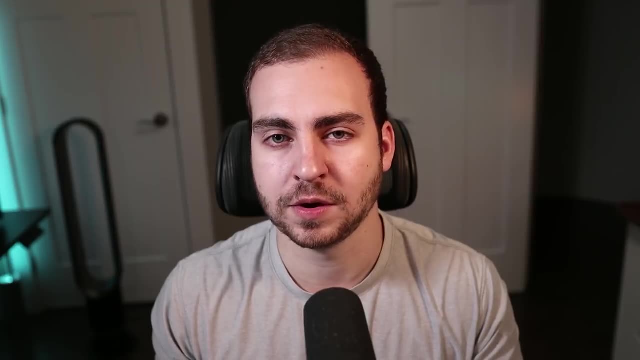 concept to go over here does not involve my computer, And this is the GIL, or the global interpreter lock. Now, this is exclusive to Python, And essentially what this says is that any thread that wants to be executing needs to acquire the interpreter lock. Now, what that? 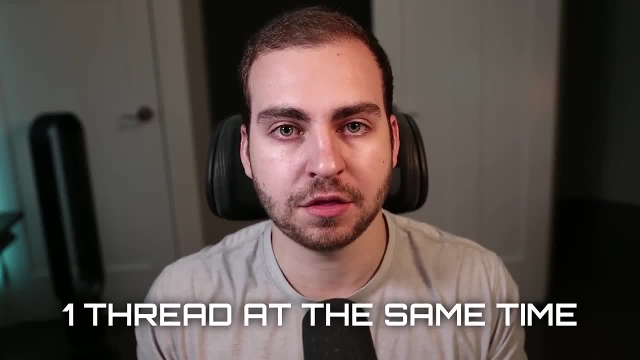 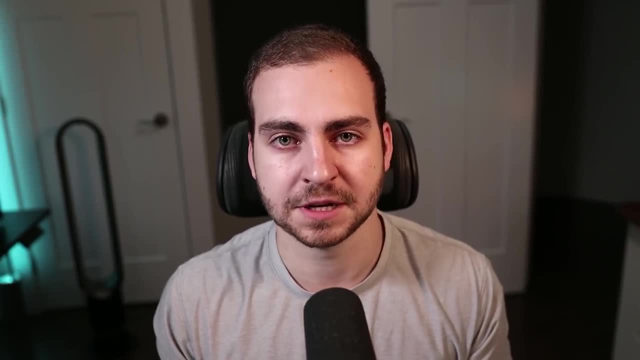 kind of technically means for you is that you can only execute one thread at the same time, even if you have multiple CPU cores on your computer. Now to better illustrate this cause: I'm sure it's a bit confusing. on your computer You have a CPU. 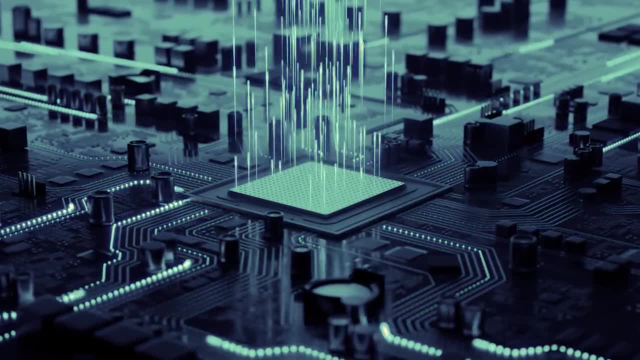 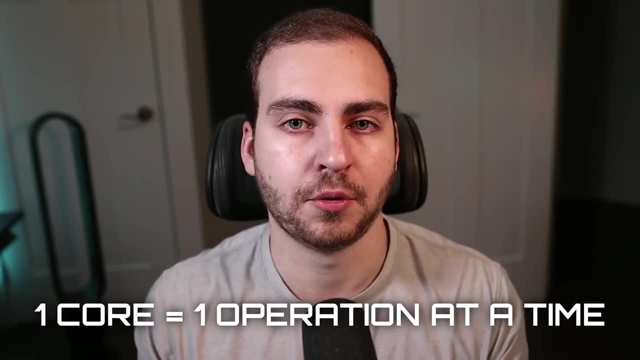 or in your computer, you have a CPU. That CPU will typically have multiple cores, two cores, four cores, eight cores, whatever it may be. Now, each one of these cores can execute one operation at a time with hyper-threading and. 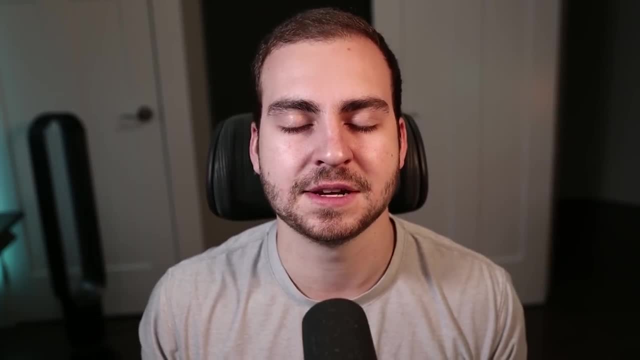 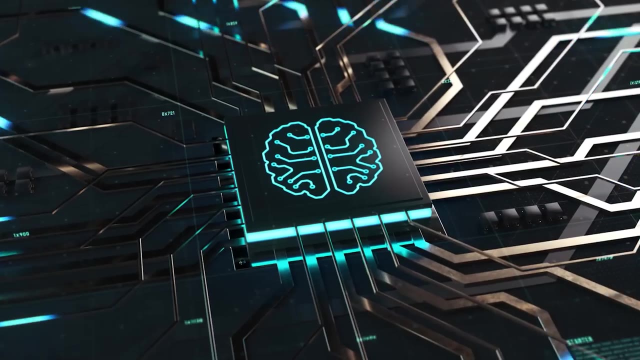 virtualization. You might be able to do a few more. I'm not going to talk about all the details there. for simplicity, Let's say each CPU core can execute one operation. Well, this is great, because that means your CPU can be working. 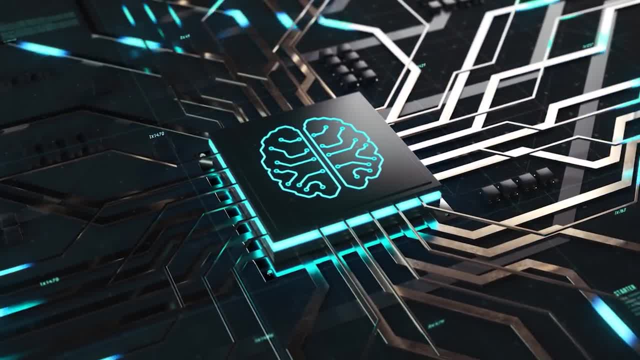 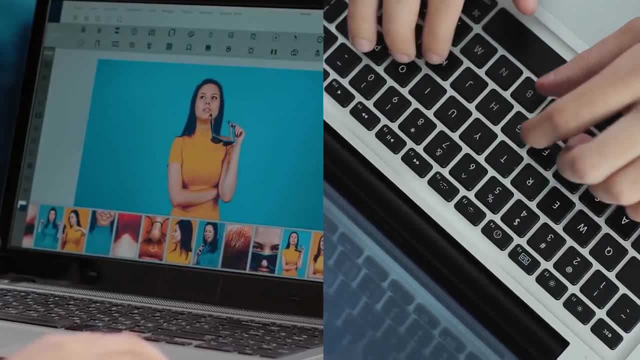 on multiple things at the same time, And if you have a complex application, it's possible that you want to be doing something like processing an image, while allowing a user to type something in, while maybe sending a request to the network. There's a ton. 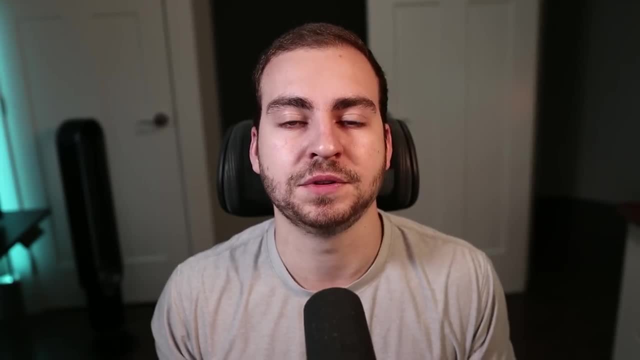 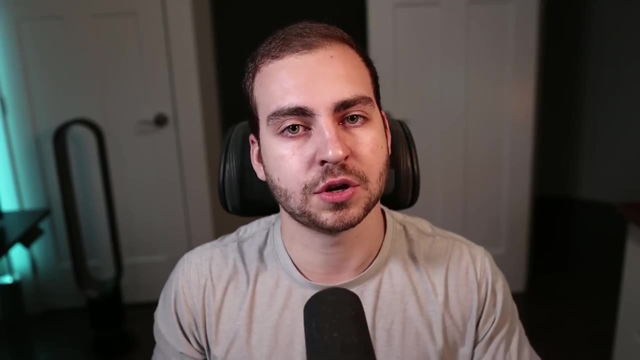 of different things you could be doing at the same time, And this is where multi-threading comes in. A thread is essentially a component of your application That's being executed by the CPU. When you start getting into larger programs, you start designing. 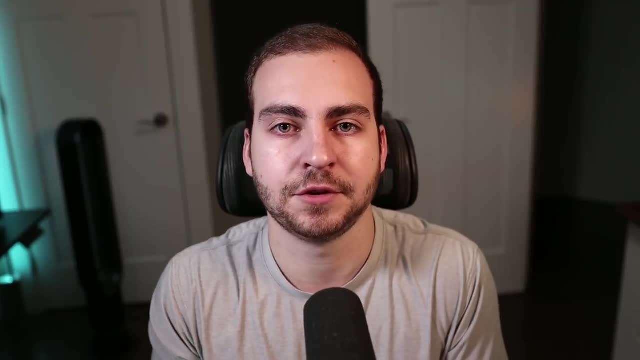 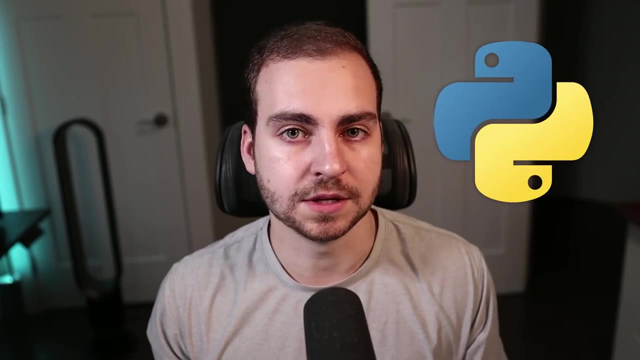 multi-threaded applications, where you have different pieces of your code separated into different threads such that they can execute at the same point in time. Now, with Python, you can do this. You can have multiple threads. The issue becomes, though, that you have this. 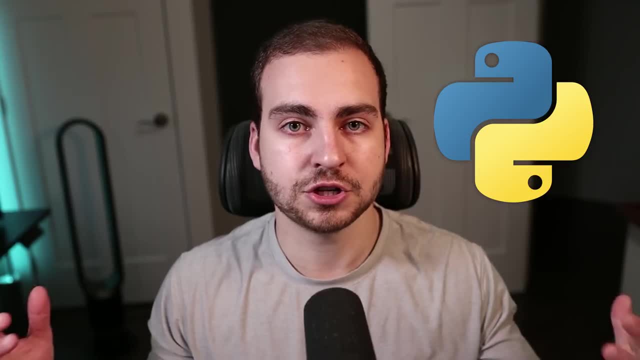 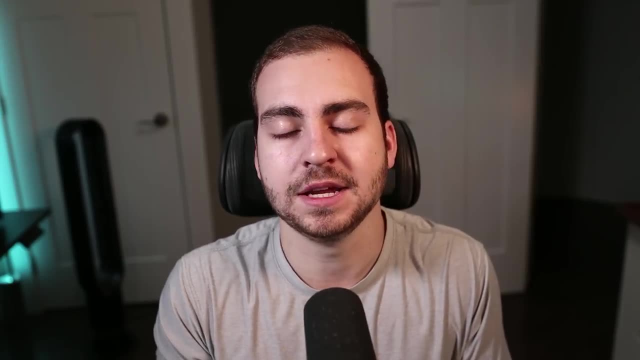 global interpreter lock. Now what that means is, even if you have a bunch of CPU cores on your computer, only one of these threads can be executing at a time. That's because this thread needs to acquire something known as a lock on the interpreter. Now I'm 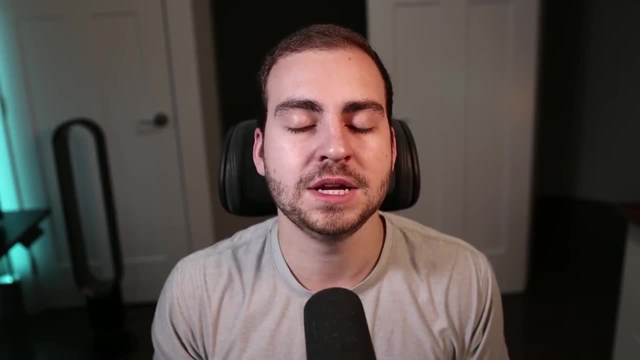 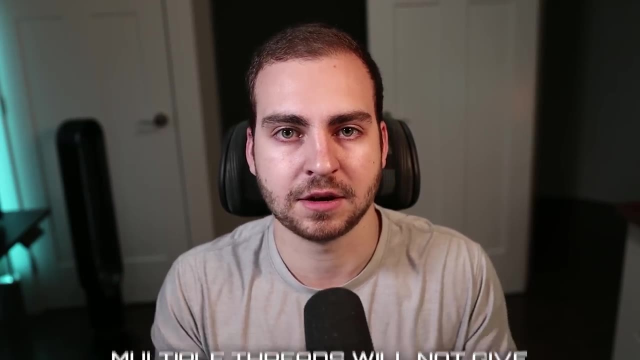 not going to discuss why this was implemented in Python, but what you need to know about this is that if you do actually have multiple threads, this is not going to give you a performance bonus in Python. It's not going to increase the speed at which you 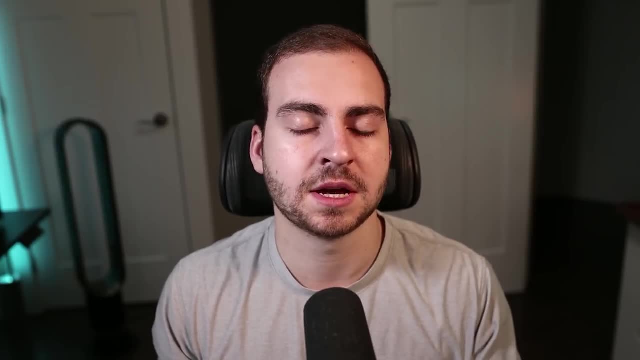 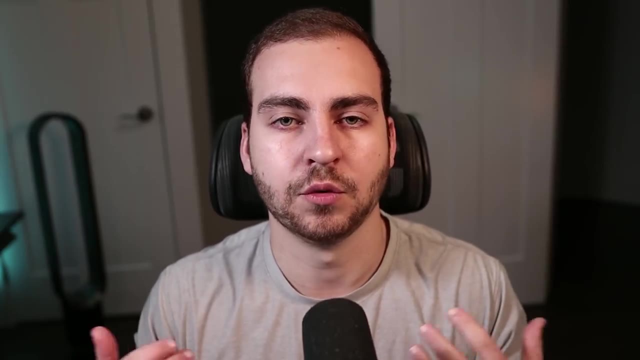 execute your code. So to give you a simple example here, let's say I want to sum the numbers from one to 100.. Well, if I was doing this in a single thread, I'd have to sum all of the numbers from one to a hundred in a.